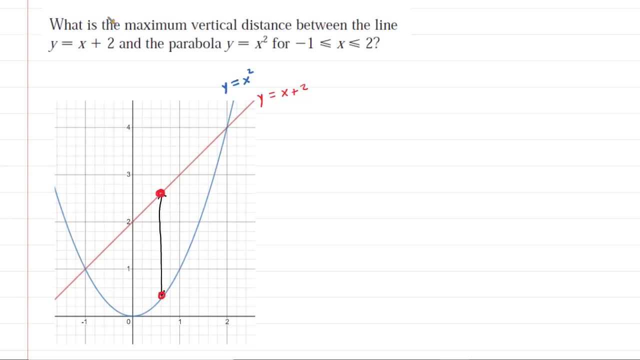 touches the red curve right there, touches the blue curve right there. That should have been blue. And we know, if we look very carefully, that the distance from that red point down to the x-axis, well, that would just be the y-coordinate of that red point. We know that the y-coordinate of that. 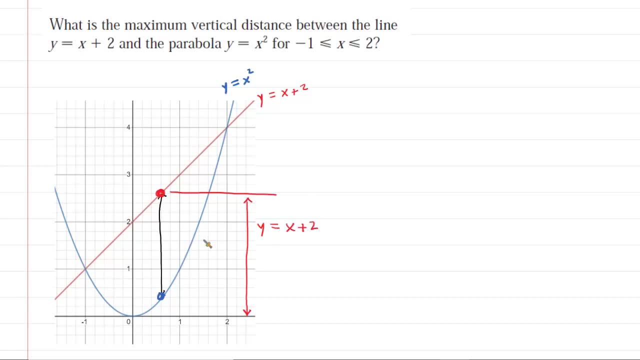 red point is x plus two. Similarly, if we look at the blue point, we know that the distance from that blue point down to the x-axis, that little distance right there would be the y-coordinate of that blue point, And we know the y-coordinate of that blue point is y is equal to x squared. 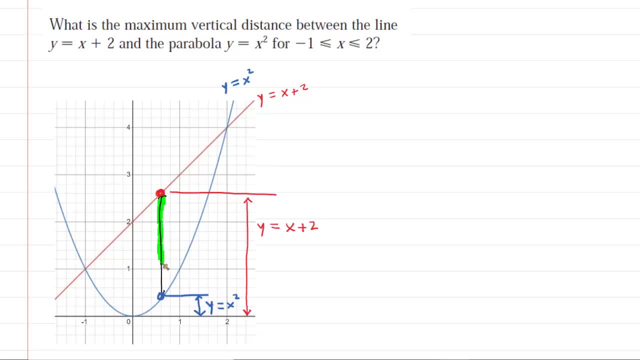 Now notice: if you wanted to represent this distance right here, then you'd have to take the vertical line in red and subtract the vertical line in blue. So what this means is that that vertical distance, which we might call v of x, would equal the length. 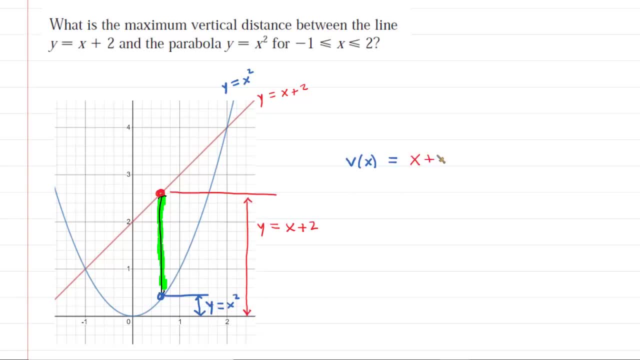 of that vertical red line, which again is x plus two, minus the length of that vertical blue line, which is x squared. So there we have an expression that represents that vertical distance in green as a function of x. Now we can simplify this a little bit. Why don't we write it in standard? 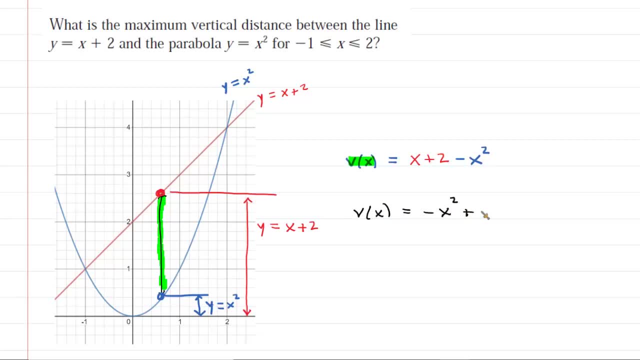 order It would be negative: x squared plus x squared x plus two. And then to find the maximum vertical distance we need the derivative. We do know that, when you're looking for a maximum, that at the maximum point the slope of the tangent 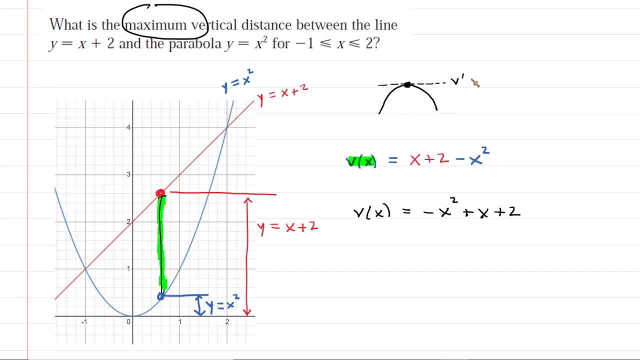 line. at that point, at that maximum, the slope is equal to zero. So this is why we're going to need to find the derivative of our function, because that derivative represents the slope of the tangent line. So here we go. x would equal the derivative of negative x. squared is just negative two x. The derivative of one x is: 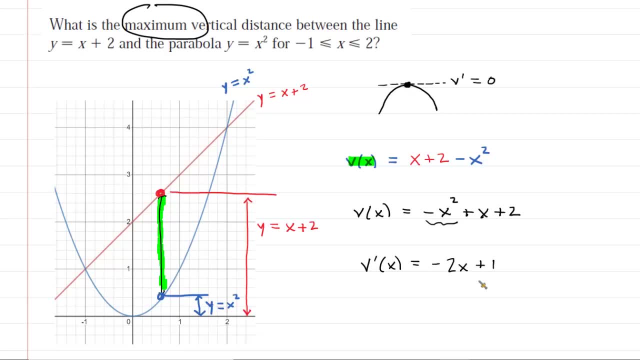 one and the derivative of that constant two is just zero. So there's the expression for your derivative. As noted, we need to set that derivative equal to zero and then solve this for x. Let's subtract the one to the other side and then divide both sides by negative two and we see. 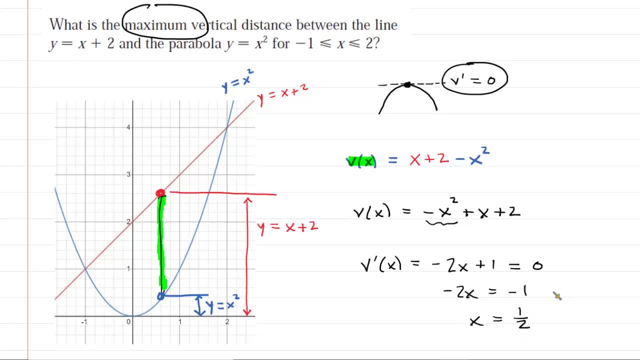 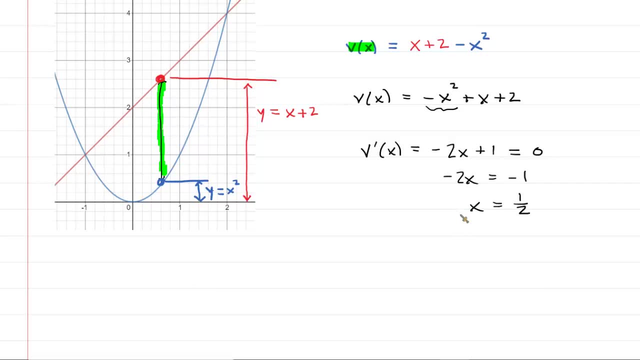 that x would equal positive one half. Now we still haven't proved that that maximizes the distance, and what we're going to do next is apply a certain test to verify that this indeed maximizes the vertical distance. And if you look, 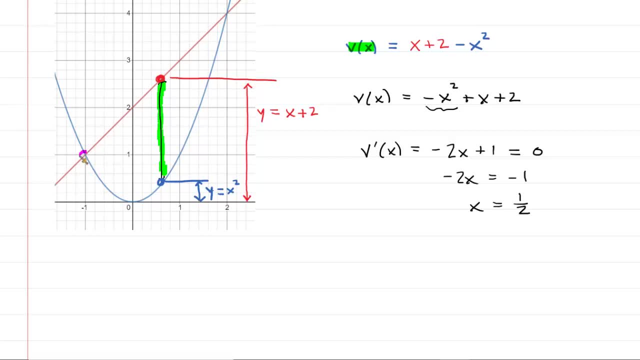 we see that the vertical distance was bounded at its lower point by negative one and at its upper point by positive two, And at those bounds it's probably obvious that the vertical distance between the curves is zero in both cases. but we can verify that by plugging negative one. 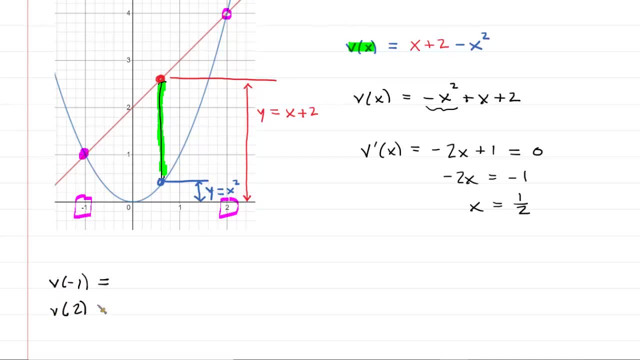 into the function, as well as plugging in positive two into the function. Notice again that negative one and positive two are the x coordinates of those bounds. If you plug negative one into this function right here, you do end up with a vertical distance of zero, as expected. And if you plug two, 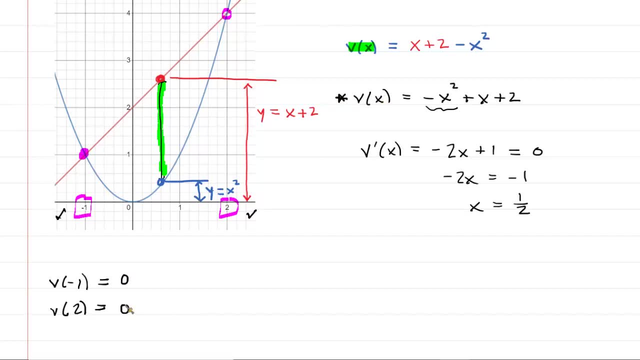 into that function. you also end up with a vertical distance of zero, as expected. But what we need to do is find the vertical distance at this so-called critical point. This was the point at which the derivative equaled zero. So we're going to do v of 1 half and again we're plugging it into the original function. 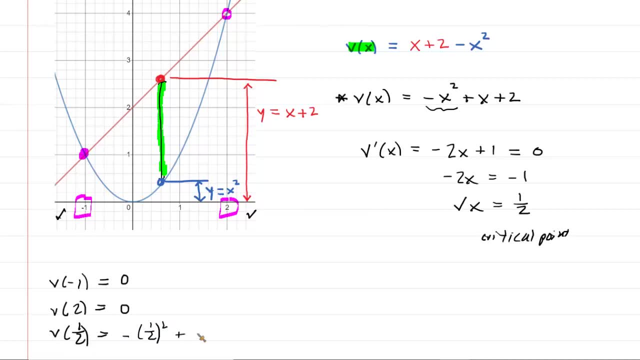 So it's going to be negative: 1 half squared plus 1 half plus 2.. And once you simplify this, you will see that that vertical distance is equal to 9 fourths. So that represents that distance. right there It is indeed the maximum distance. 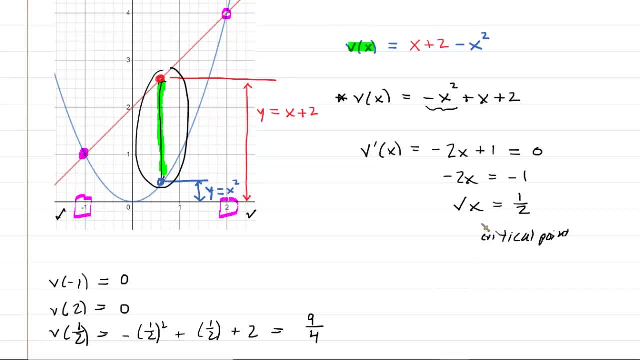 How do we know it's a maximum? Because we know that at that x value at x is equal to 1, half the slope of the tangent line was equal to 0. So that indeed represents the maximum point. Let's just make sure that we have answered the question. 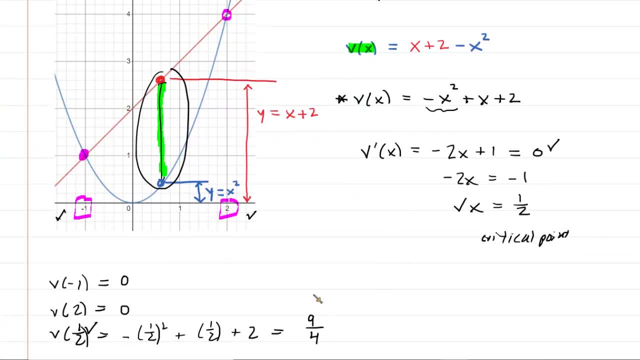 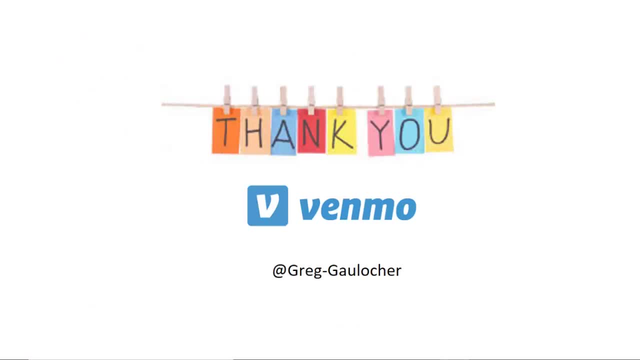 It says what is the maximum vertical distance? Yeah, indeed, it is 9 fourths, So that is the correct answer to the question. Thanks for taking the time to watch the video. If you're interested in making a small donation to my cause, I would greatly appreciate it. If not, no worries, Thank you. Thanks for taking the time regardless.